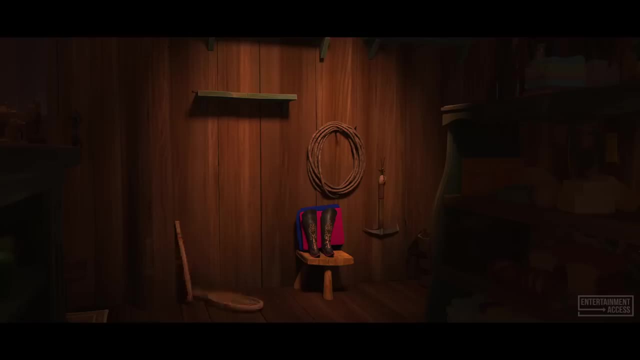 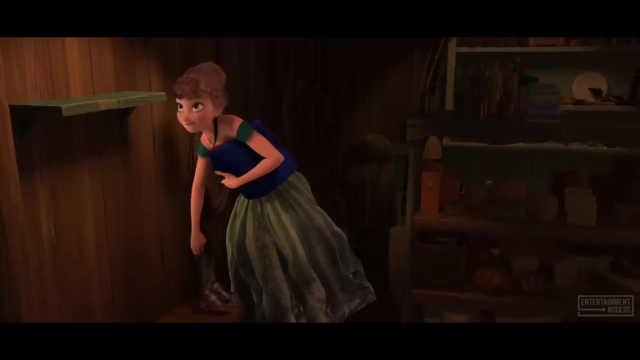 That would be in our winter department. Oh, Oh, Um. I was just wondering: has another young woman- the queen perhaps, I don't know- Pass through here? Only one crazy enough to be out in this storm? is you, dear? 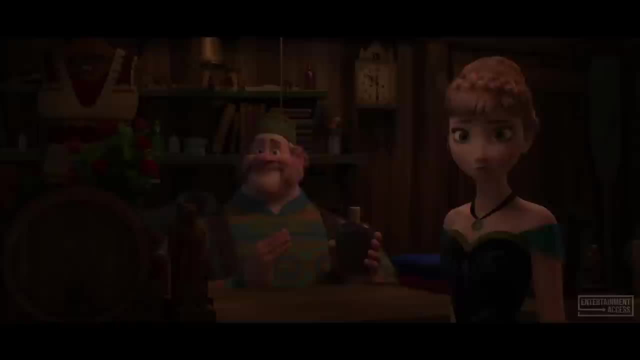 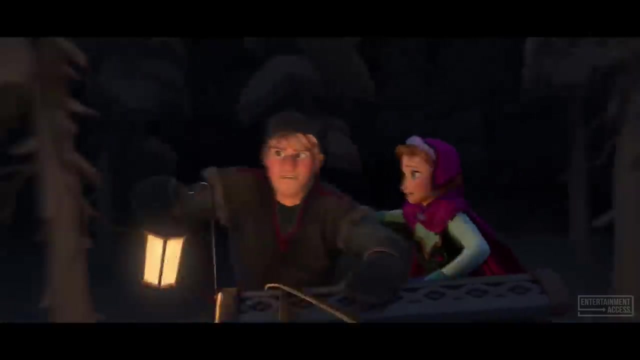 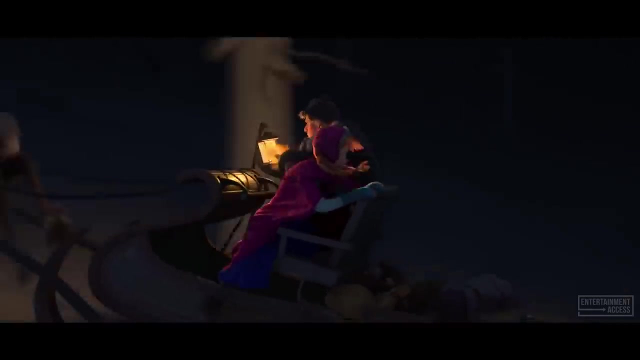 You and this fellow Woo-hoo, Big summer blowout. Sven, go Go. What are they? Wolves, Wolves, What do we do? I got this. You just don't fall off and don't get eaten. But I want to help. 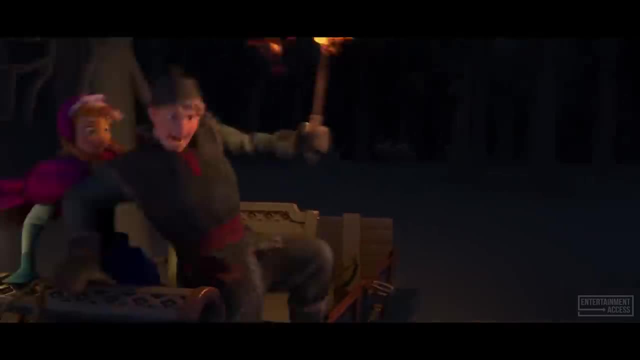 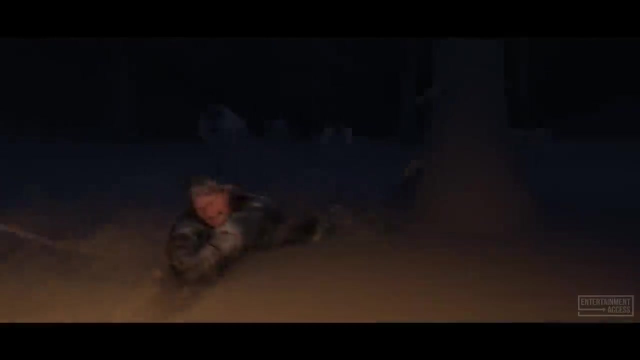 No, Why not? Because I don't trust your judgment, Excuse me. Who marries a man she just met? It's true love. Whoa, Whoa, Whoa. Christopher, It's Krista Ow Ah. 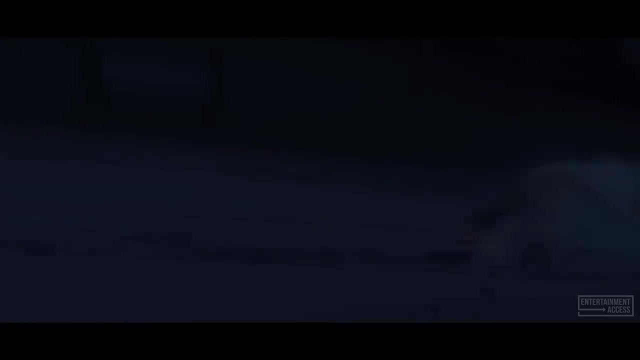 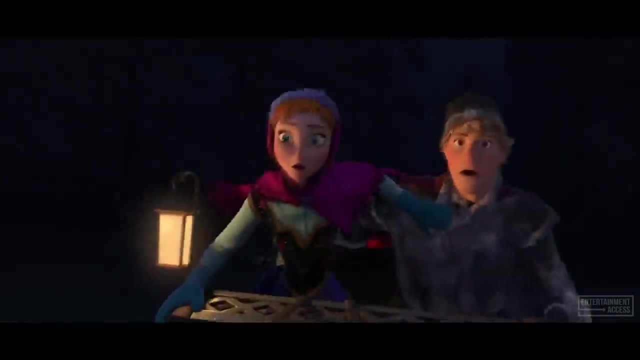 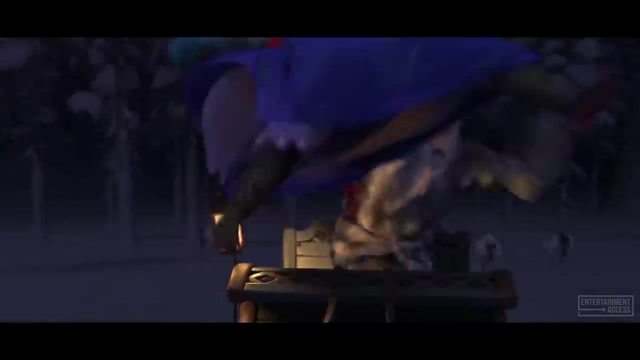 Duck. Ah, You almost set me on fire, But I didn't Get ready to jump Sven. You don't tell him what to do. Hey, I do Woo Jump Sven. Ah, Ah, Ah. 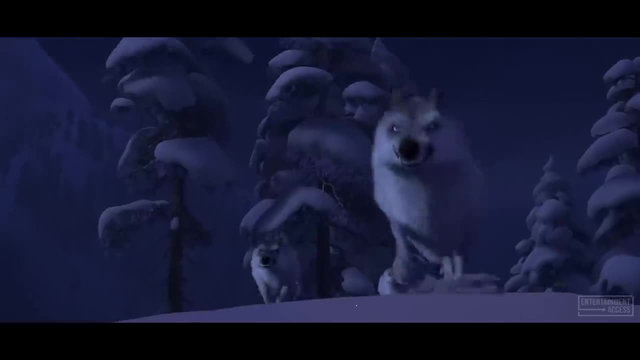 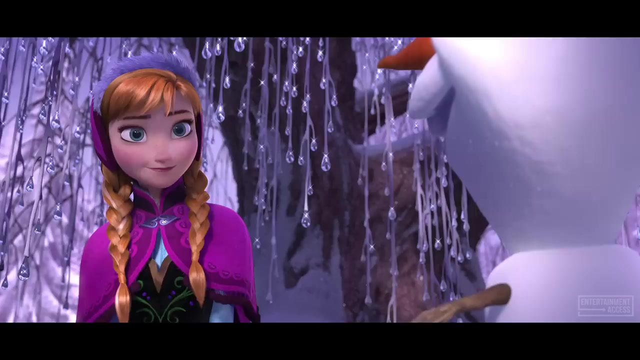 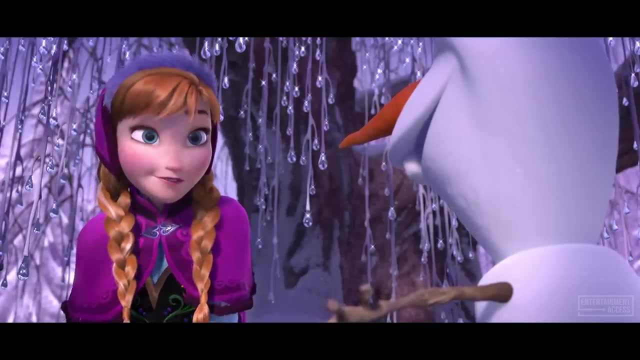 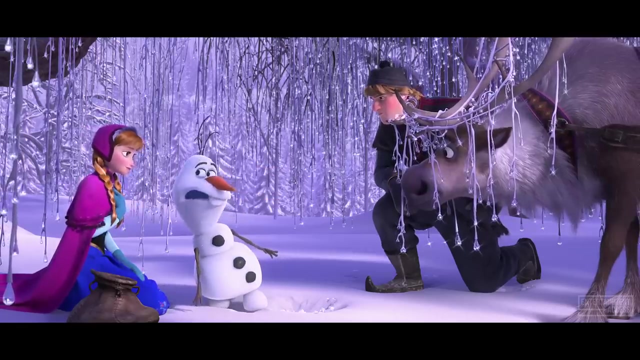 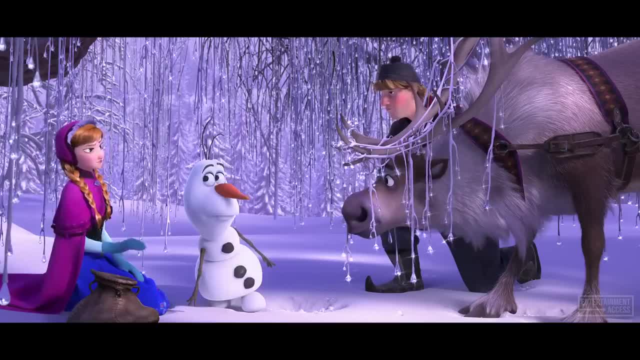 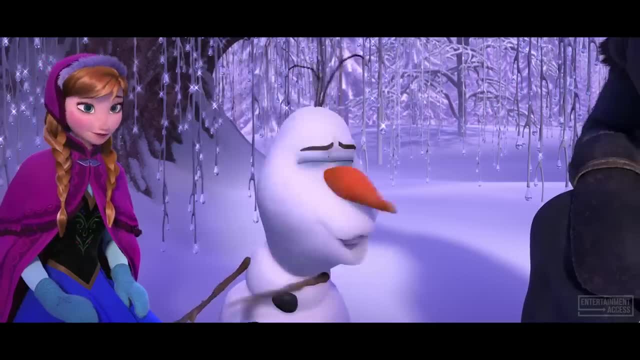 That's Sven, Uh-huh. And who's the reindeer, Sven? Oh, Oh, OK, Make things easier for me. Oh, look at him trying to kiss my nose. I like you too, Olaf. 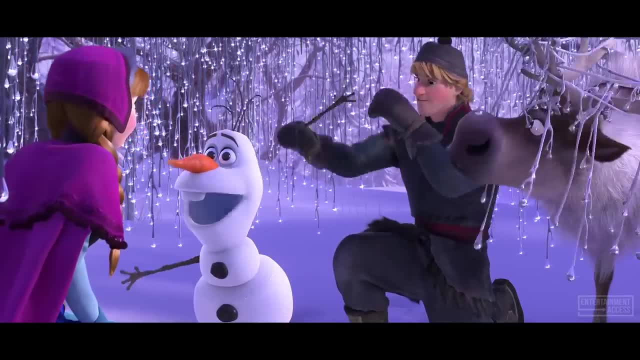 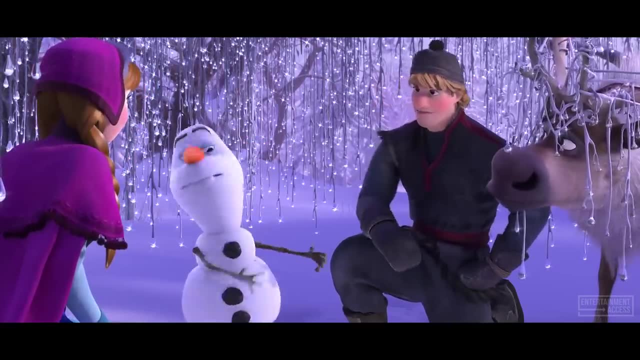 Did Elsa build you? Yeah, why Do you know where she is Fascinating? Yeah, why Do you think you could show us the way? Yeah, why. How does this work? Ow, Stop it, Sven. I'm trying to focus here. 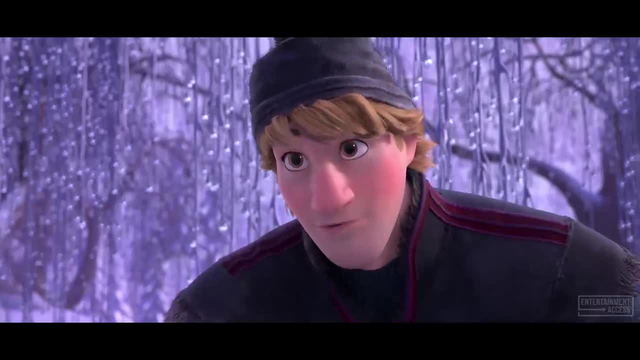 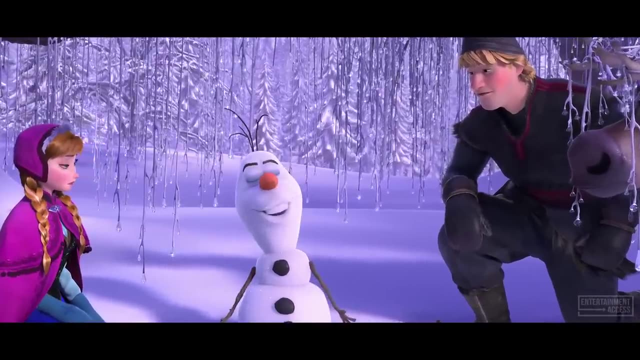 Yeah, why? I'll tell you why We need Elsa to bring back summer. Summer, Mm-hmm. Oh, I don't know why, but I've always loved the idea of summer and sun and all things hot Really. 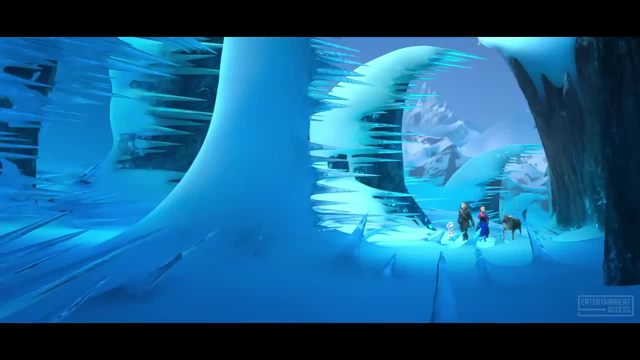 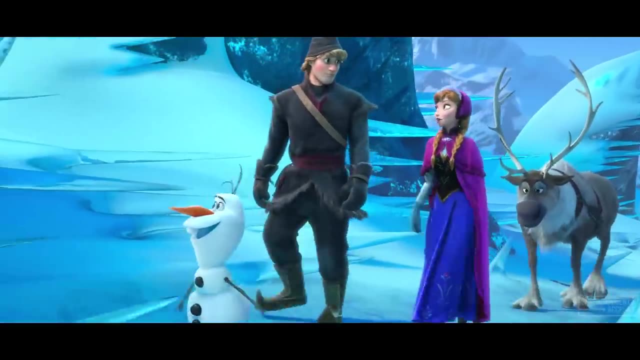 I'm guessing you don't have much experience with heat? Nope, So how exactly are you planning to stop this weather? Oh, I am going to talk to my sister. That's your plan. My ice business is riding on you. talking to your sister? 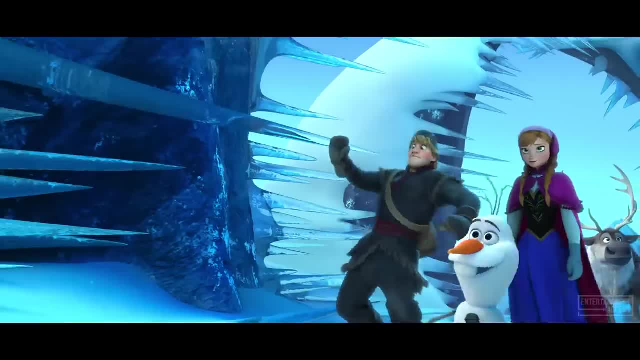 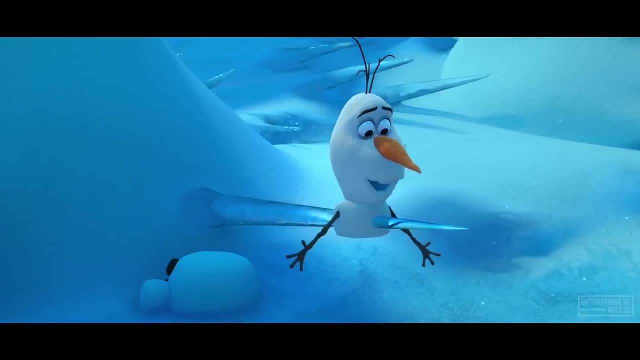 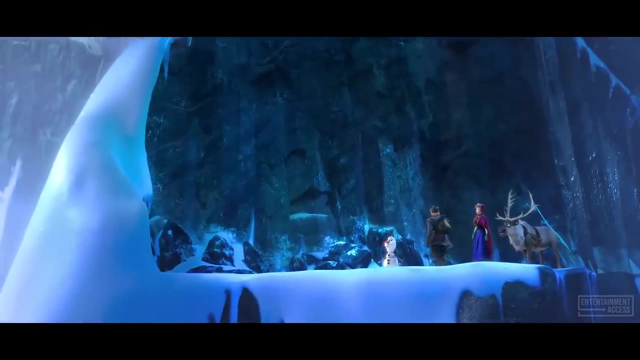 Yep, So you're not at all afraid of her. Why would I be? Yeah, I bet she's the nicest, gentlest, warmest person ever. Oh, look at that, I've been impaled. What now? It's too steep. 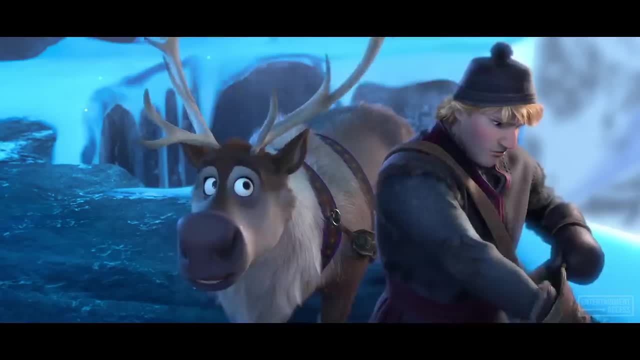 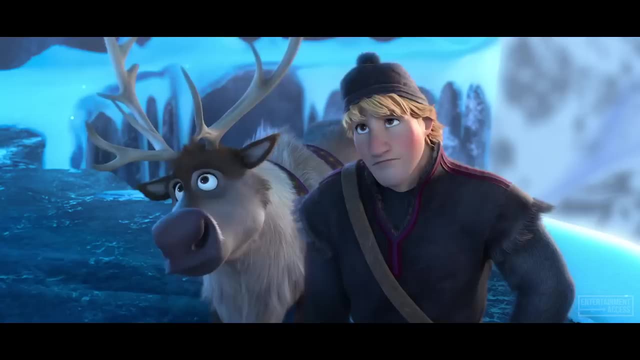 I've only got one rope and you don't know how to climb mountains. Says who. What are you doing? I'm going to see my sister. You're going to kill yourself. I wouldn't put my foot there. You're distracting me. 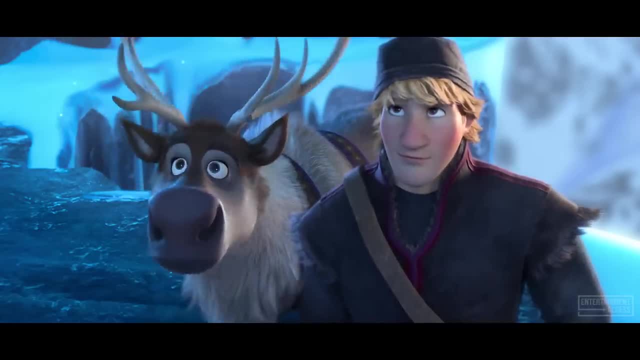 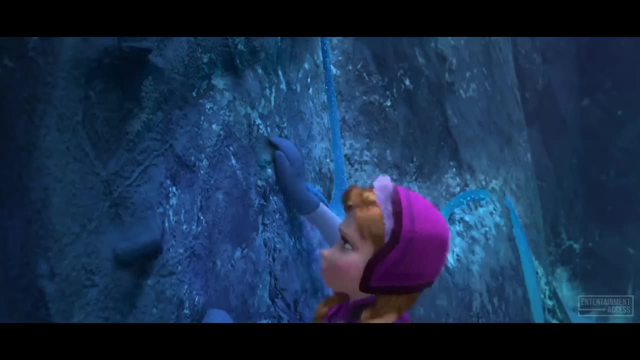 Or there. How do you know? Elsa even wants to see you. All right, I'm just blocking you out because I've got to concentrate here. You know, most people who disappear into the mountains want to be alone. Nobody wants to be alone. 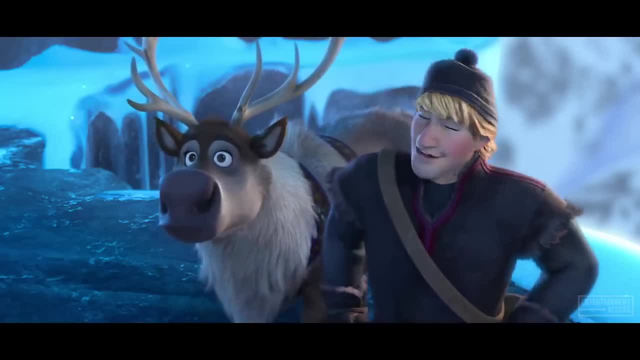 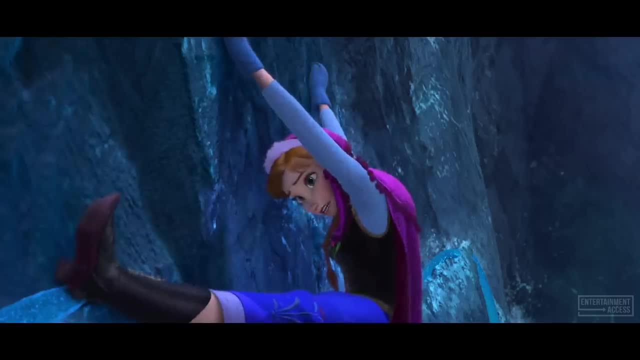 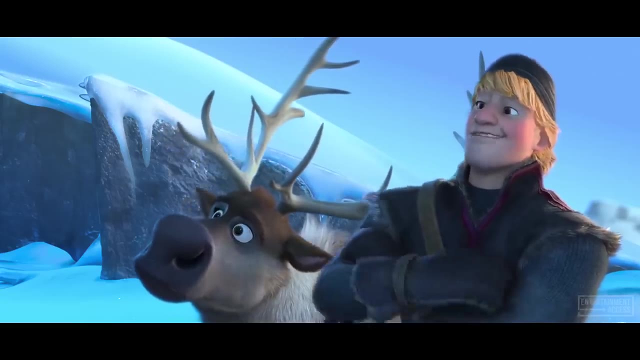 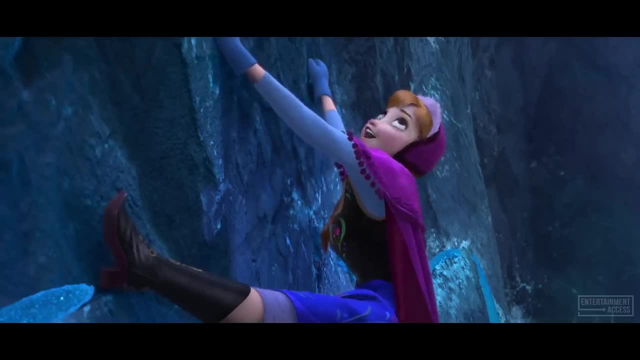 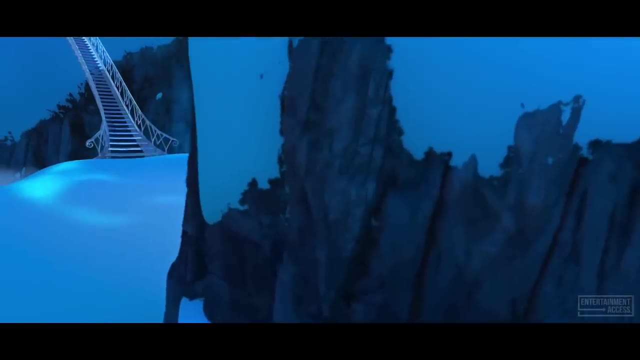 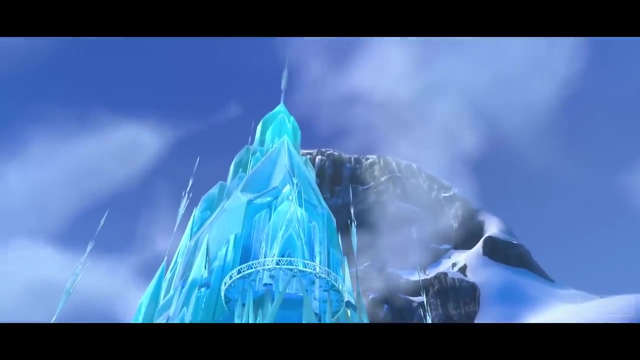 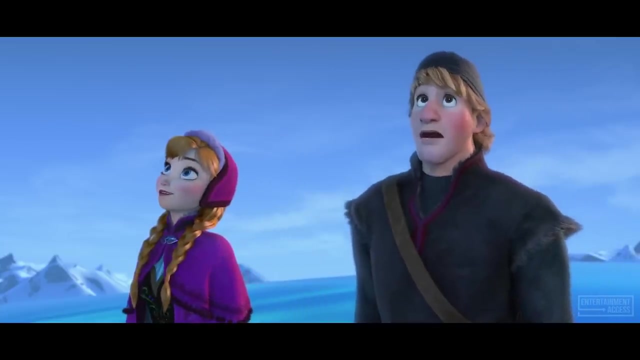 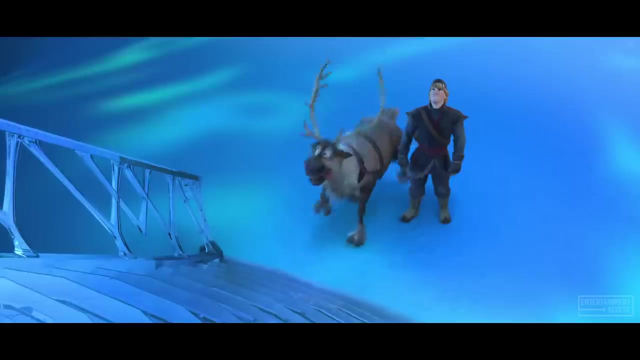 but I found a staircase that leads exactly where you want it to go. Ha ha, Thank goodness, Catch Thanks. That was like a crazy trust exercise. I've got you. Now that's ice. I might cry: Go ahead, I won't judge. 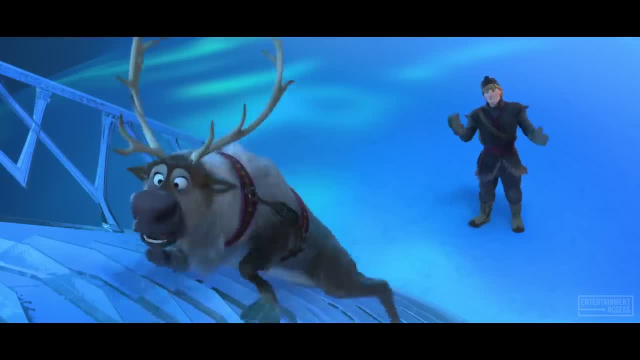 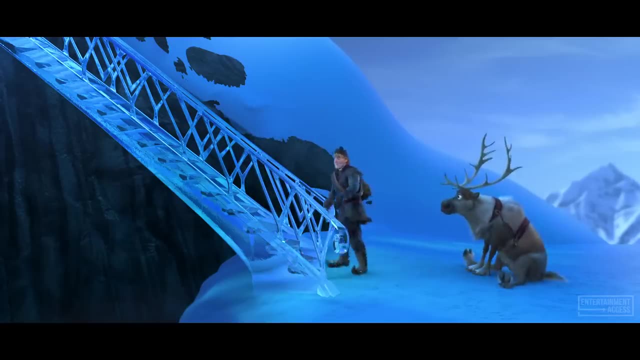 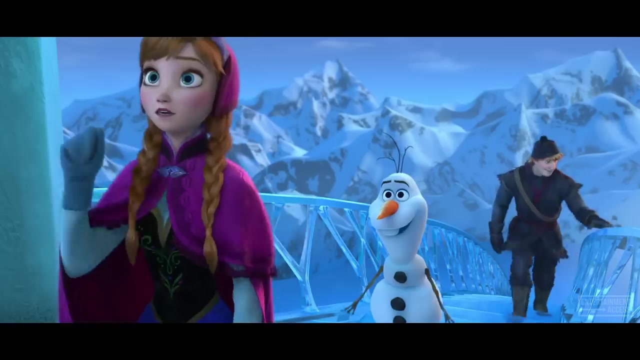 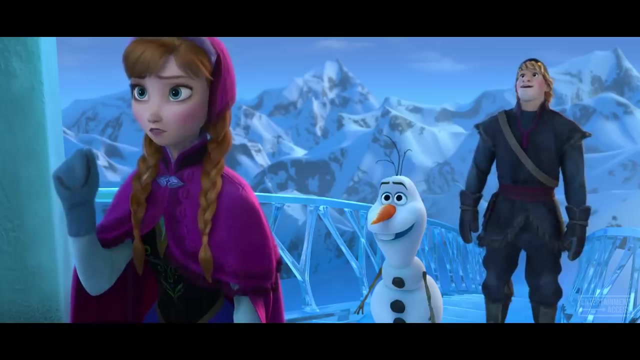 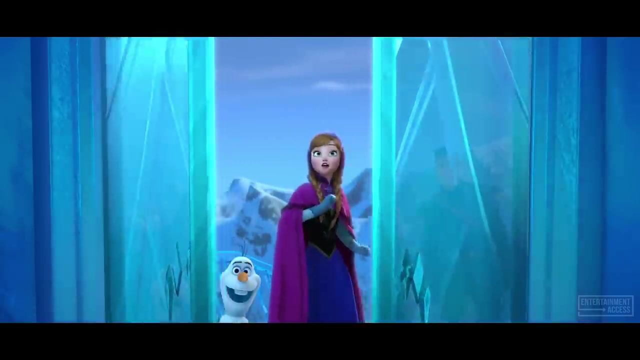 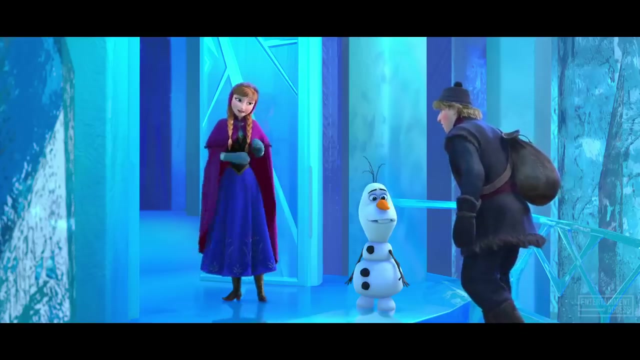 All right, take it easy, boy, Come here, I got you. Okay, you stay right here, buddy, Flawless. Okay, knock, just knock. why isn't she knocking? do you think she knows how to knock it opened? that's a first. oh, you should probably wait out here. what last time i introduced her? 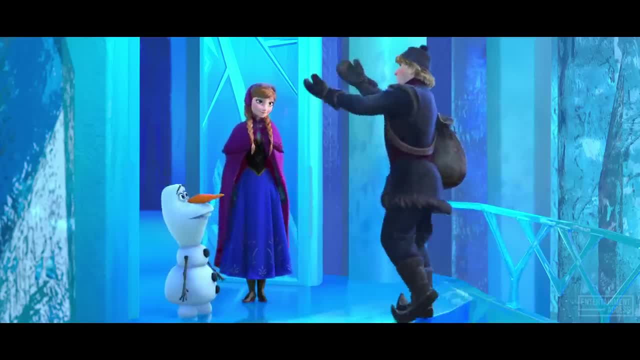 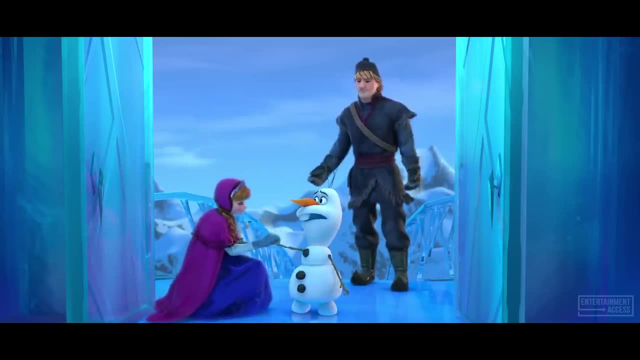 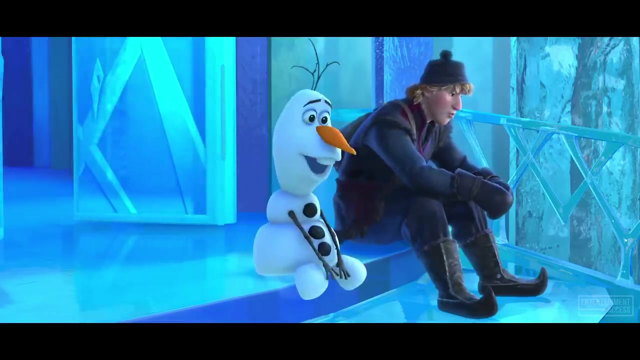 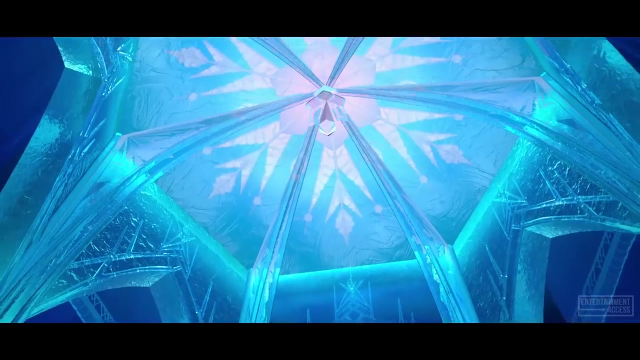 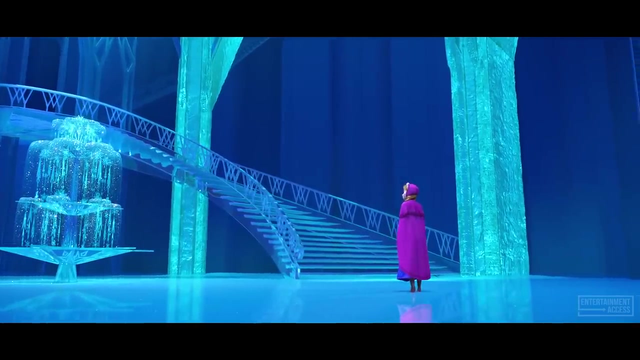 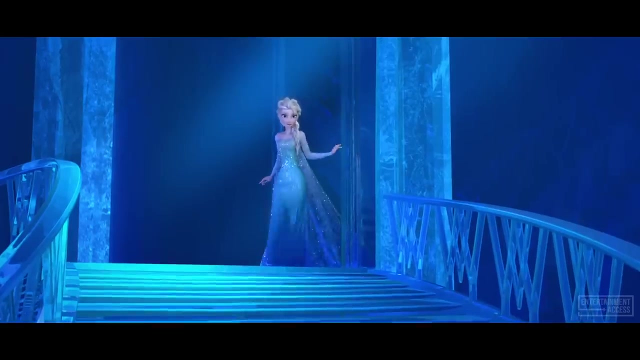 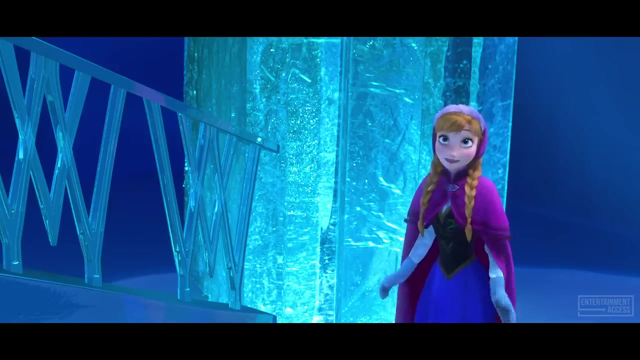 to a guy. she froze everything, but but oh, come on, it's a palace made of ice. ice is my life. bye, Sven, you too. Olaf, me, just give us a minute, okay, one, two, three, four. Elsa, it's me. Anna, whoa, Elsa, you look different. it's a good difference, and this place, it's. 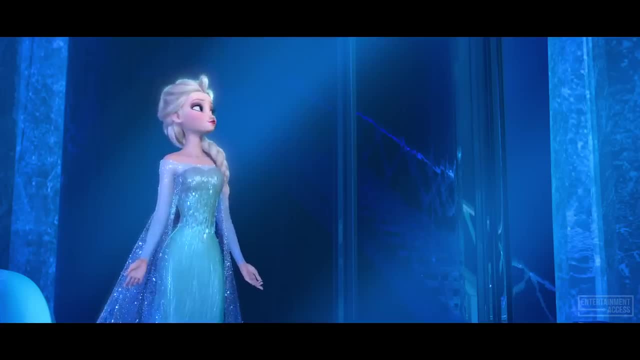 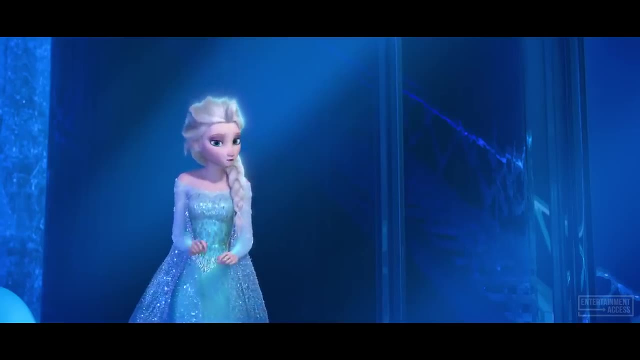 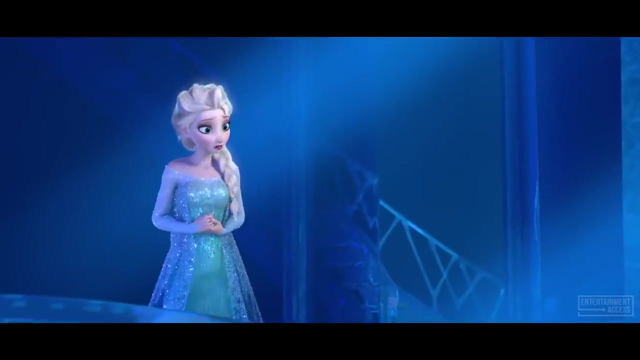 amazing. thank you. I never knew what I was capable of. I'm so sorry about what happened. if I'd have known. oh no, it's okay, you, you don't have to apologize, but you should probably go, please. but I just got here. you belong down in Arendelle, so do you? 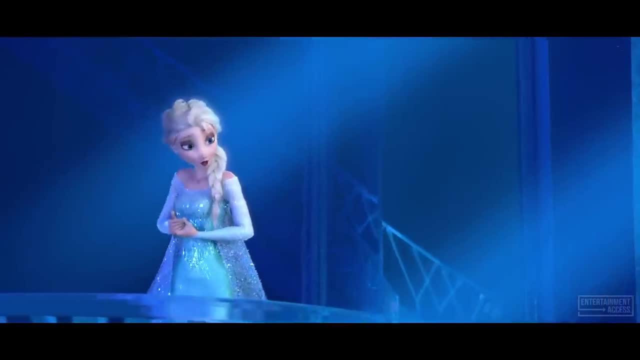 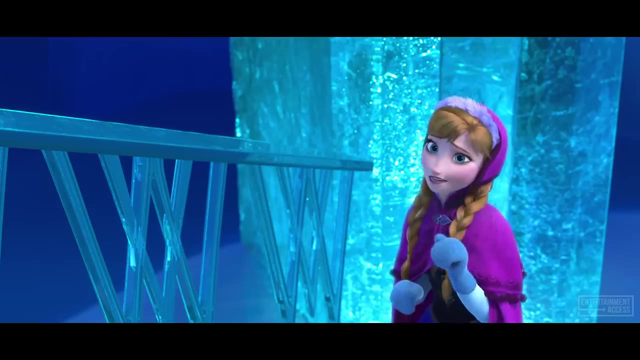 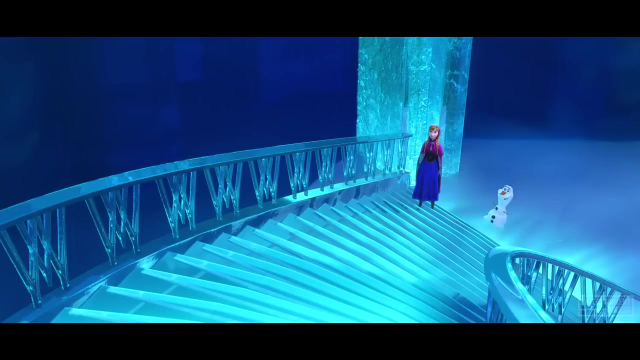 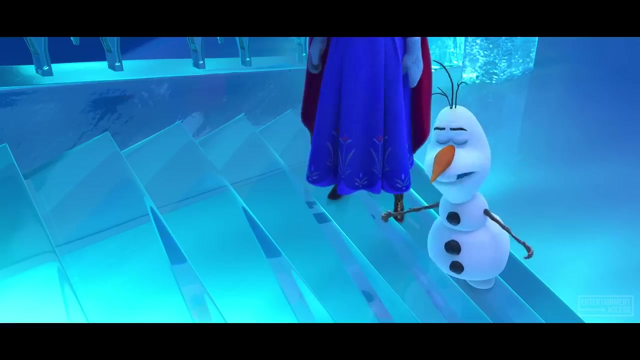 no, Anna, I belong here alone, where I can be who I am without hurting anybody. actually, about that. wait, what is that? hey, I'm Olaf and I like warm hugs. Olaf, you built me, remember that, and you're alive. yeah, um, I think so. he's just like the one we built as kids. 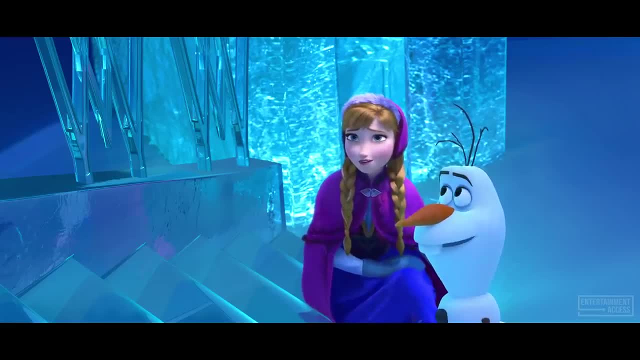 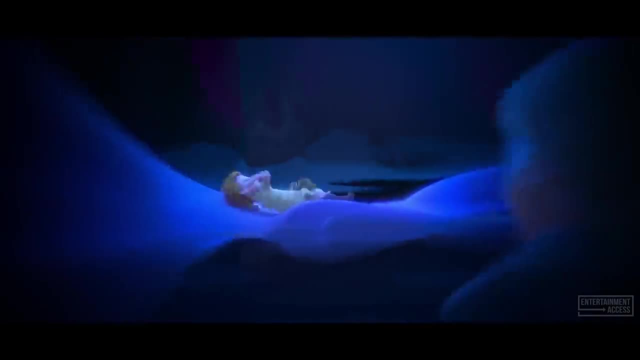 yeah, so we were so close. we can be like that again. no, we can't. goodbye, Anna Elsa, wait, no, I'm staying here. WAIT, I CAN'T GO TO THE PALE 2, ELSA, I JUST CAN'T GO TO THE PALE 2. HAHA, top rock. 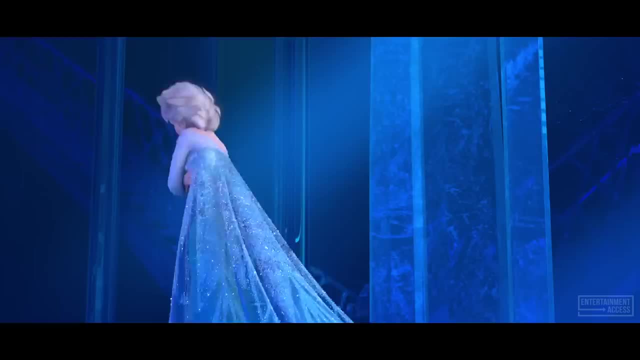 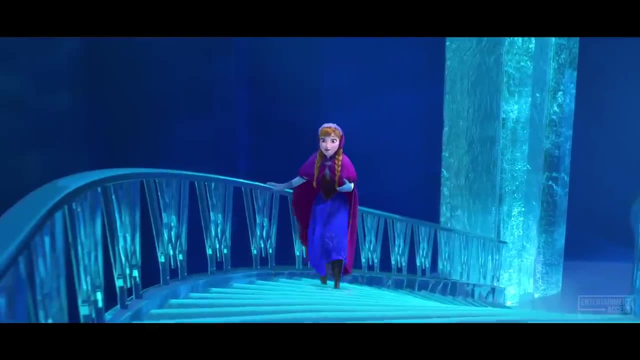 Elsa, you seem to be feeling it again. bottom rock, corner of the 알아, top rock, just trying to protect you. You don't have to protect me, I'm not afraid. Please don't shut me out again. Please don't slam the door. You don't have to keep your distance anymore. 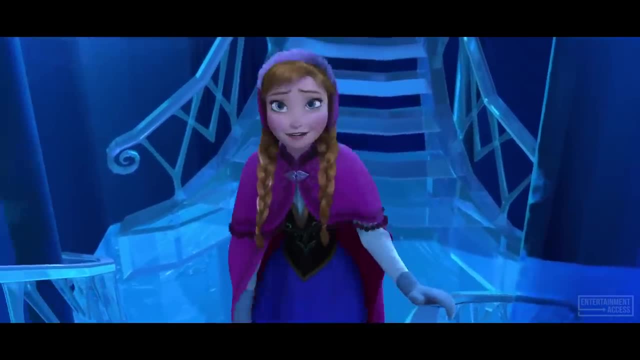 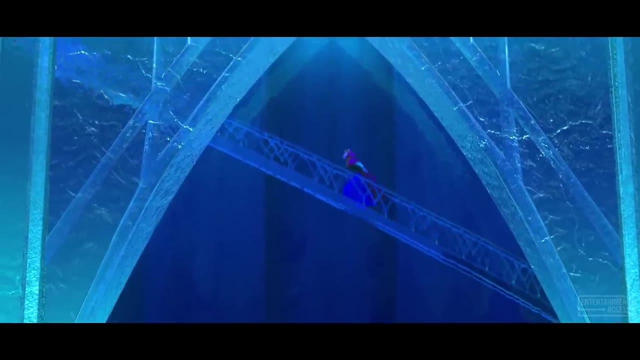 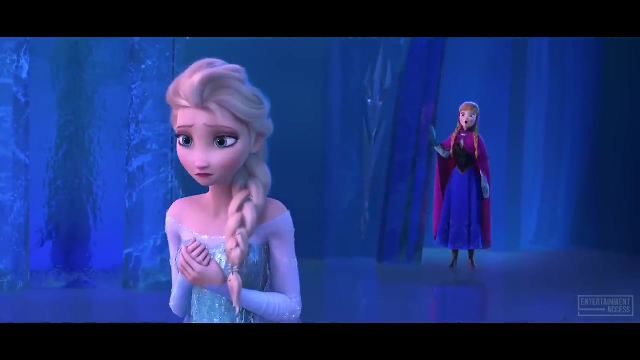 Cause. for the first time in forever, I finally understand. For the first time in forever, we can fix this hand in hand. We can head down this mountain together. You don't have to live in fear Cause. for the first time in forever, I will be right here. Anna, please go back home. 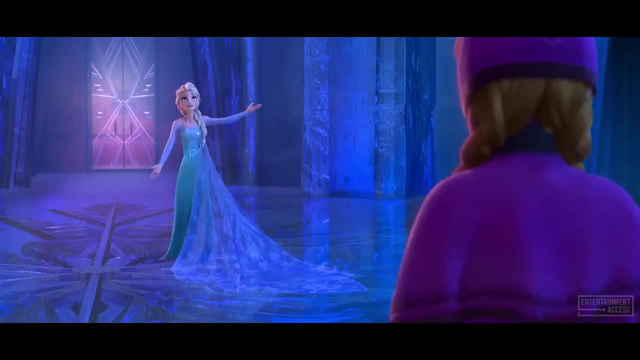 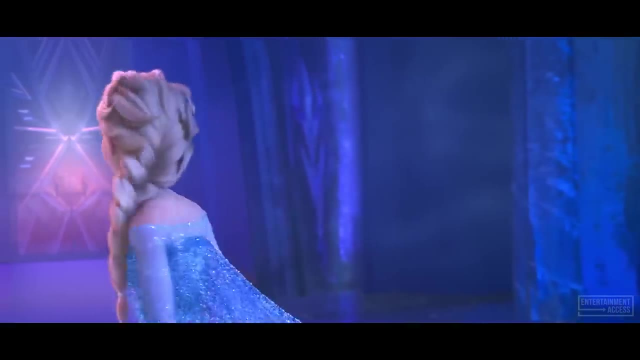 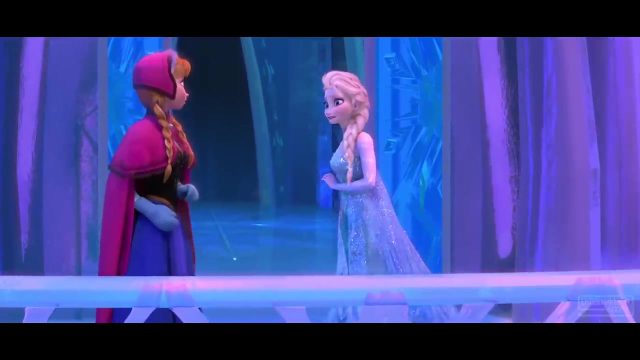 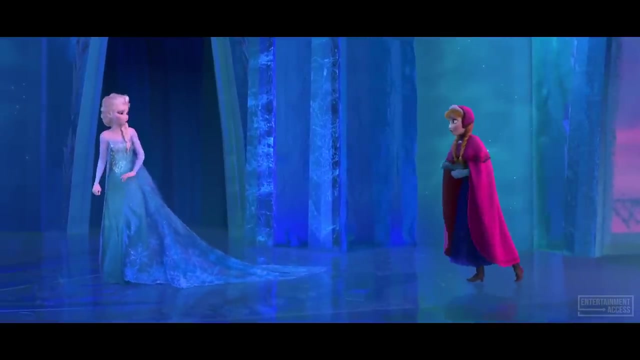 Your life awaits. Go, enjoy the sun and open up the gates. Yeah, but I know you mean well, but leave me be. Yes, I'm alone, but I'm alone and free. Just stay away and you'll be safe From me. Actually, we're not. What do you mean? you're not. I get the feeling you don't know. 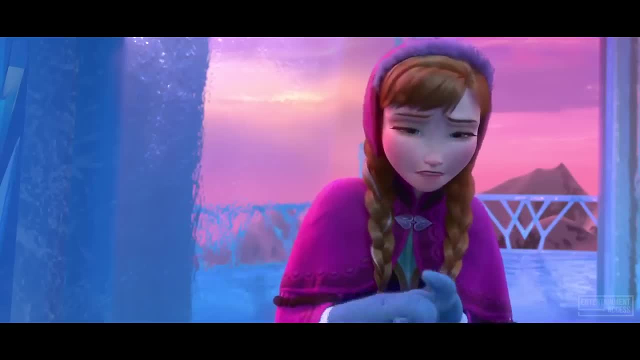 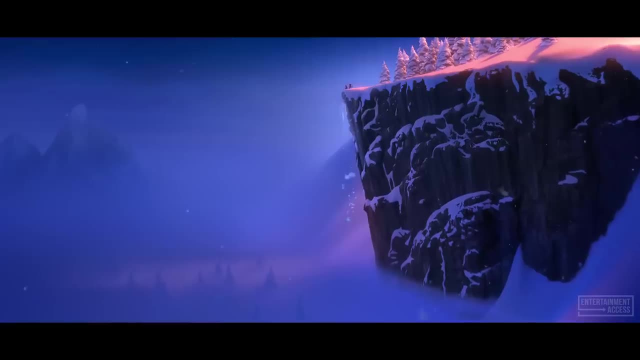 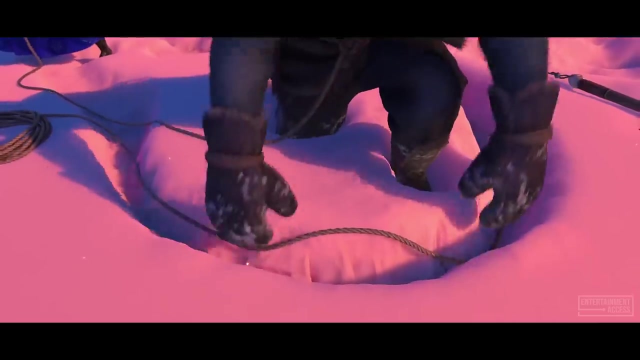 What do I not know? Our angels in deep, deep, deep, deep snow. It's a hundred foot drop, It's 200.. Ow, What's that for? I'm taking a snow anchor. Okay, What if we fall? There's 20 feet of fresh powder down there. It'll be like landing on a pillow, Hopefully. 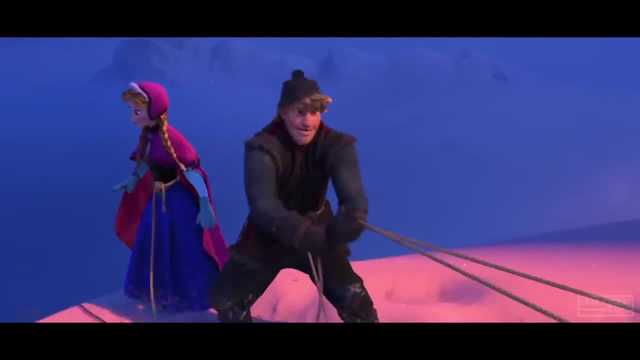 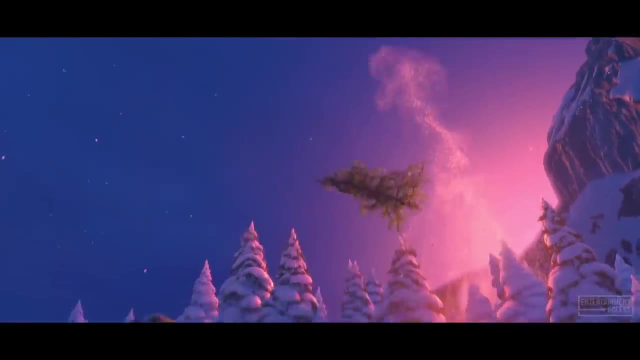 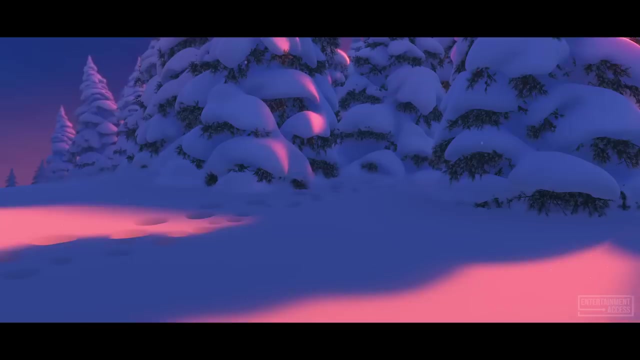 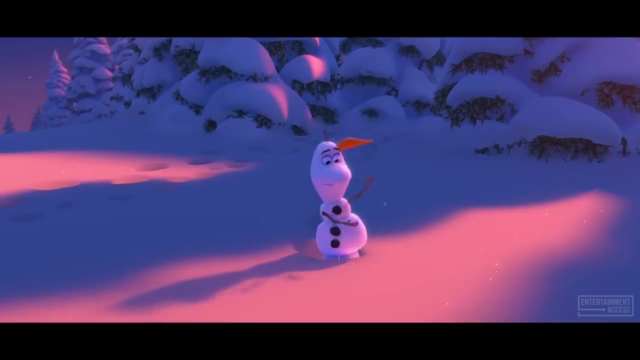 Hey Anna, On three. Okay, One, You tell me when I'm ready to go. Two, I was born ready. Yes, Calm down. What the That happened, Man, am I out of shape? There we go. Hey Anna, Sven, Where'd? 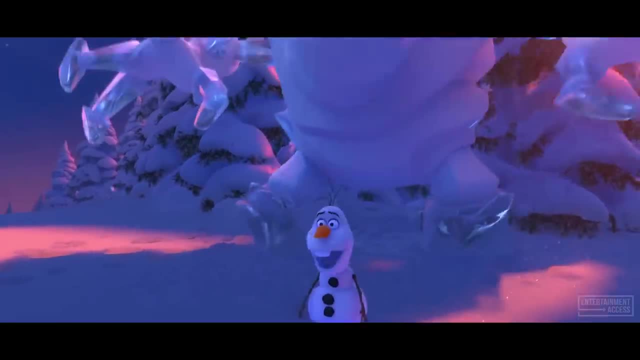 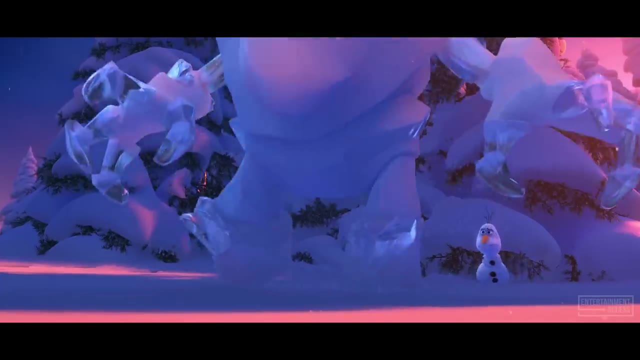 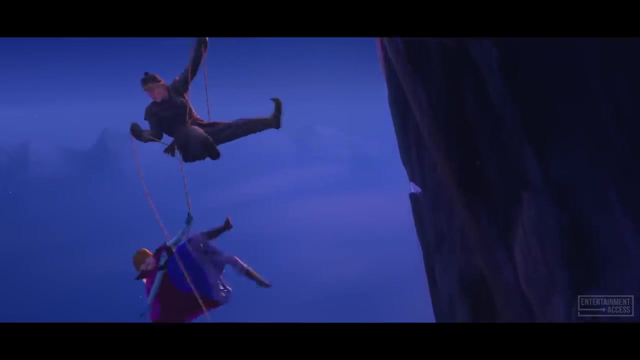 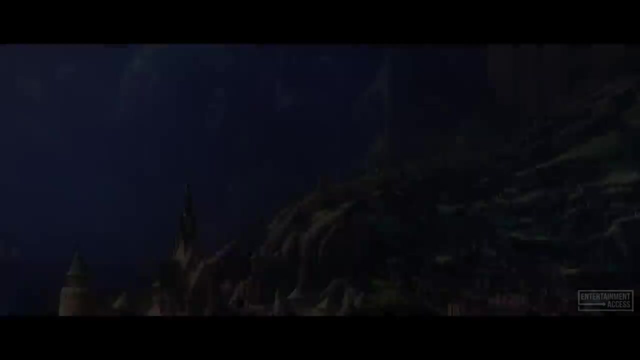 you guys go. We totally lost Marshmallow back there. Hey, we were just talking about you. All good things, All good things. No, This is not making much of a difference. is it Summer in the city of Arendelle? It couldn't be warmer, It couldn't be sunnier, but that's about.